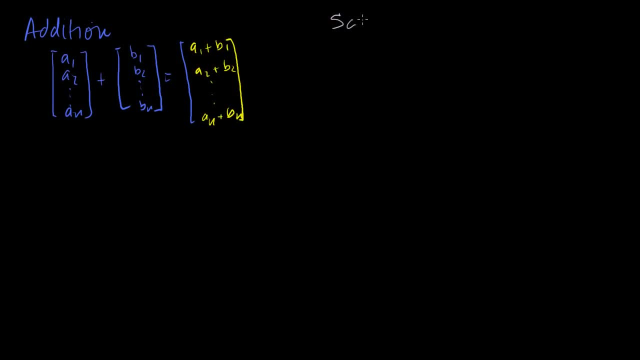 We also know about scalar multiplication, Or maybe we should just call it scaling Multiplication, And that's the case. Look, if I have some real number c and I multiply it times some vector: a1,, a2, all the way down to an we define. 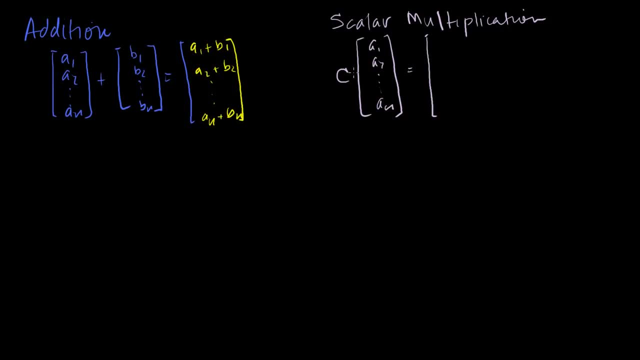 scalar multiplication of a vector to be some scalar times this vector will result in essentially this vector where each of its components are multiplied by the scalar ca1, ca2, all the way down to ca2.. baAient, c, bn. 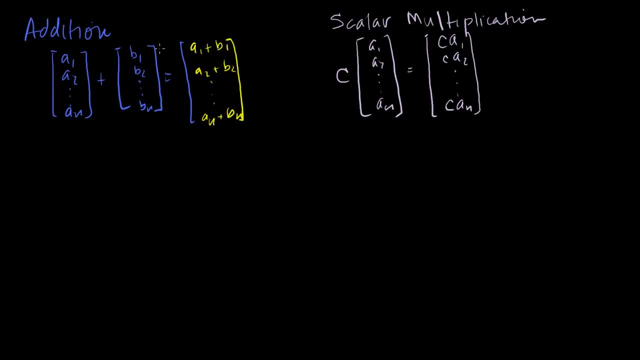 And so, after seeing these two operations, you might be tempted to say, gee, wouldn't it be nice if there was some way to multiply two vectors? This is just a scalar times a vector. You're just scaling it up and that's actually the actual. 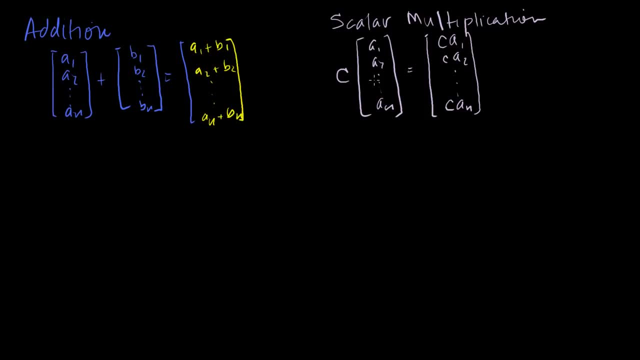 effect of what it's doing. if you visualize it IN less, in three dimensions or less, It's actually scaling the size of the vector And we actually haven't defined the size very precisely just yet. But you understand at least this operation. 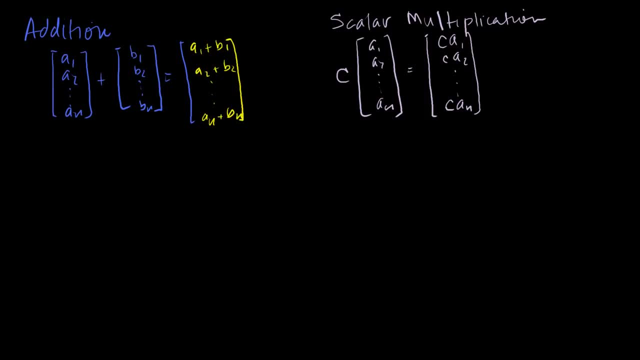 For multiplying vectors or taking the product there's, put it into the left area. You have to do a, for example, I'm going to define one of them in this video and that's the dot product. And you signify the dot product by saying a, dot b. 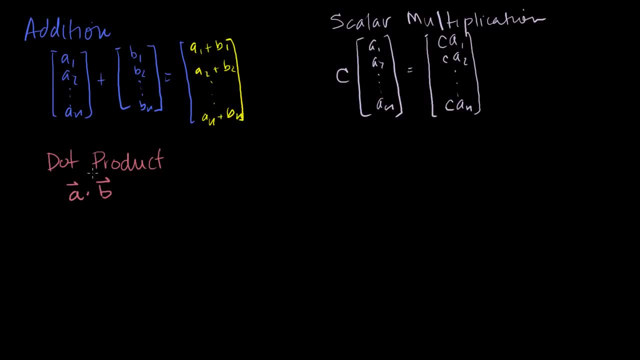 So they borrowed one of the types of multiplication notations that you saw, but you can't write a cross here. That'll be actually a different type of vector multiplication. So the dot product is almost fun to take because it's mathematically pretty straightforward, unlike the 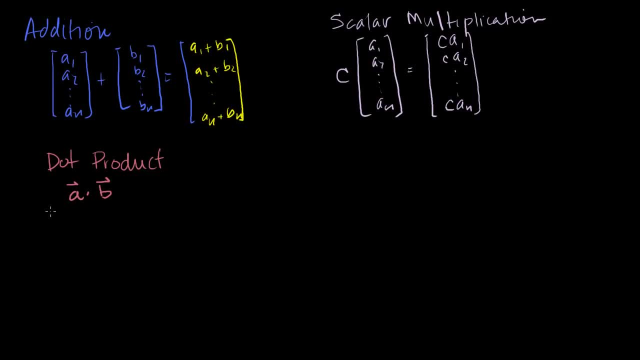 cross product But it's fun to take and it's interesting because it results. so this is: a1, a2, all the way down to an. That vector dot my b vector. b1,, b2, all the way down to bn. 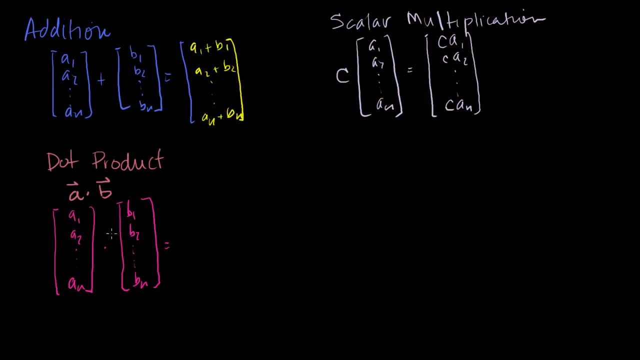 is going to be equal to the product of each of their corresponding components. So a1, b1. Added together, plus a2, b2,, plus a3, b3, plus all the way to an bn. So what is this? 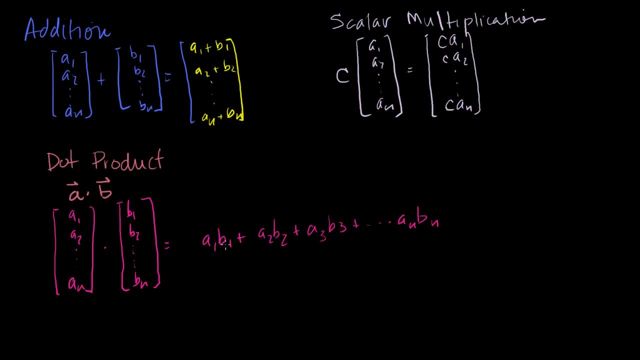 Is this a vector? Well, no, this is just a number. This is just going to be a real number. You're just taking the product and adding together a bunch of real numbers. So this is just going to be a scalar, a real scalar. 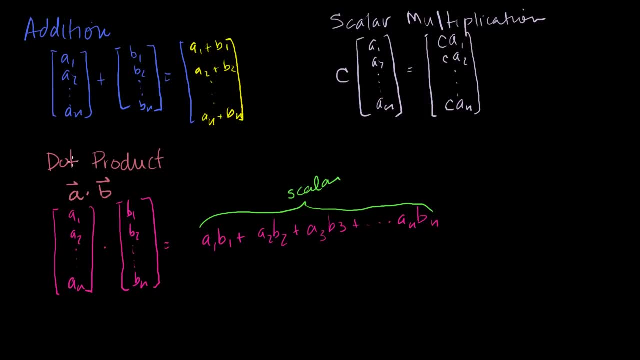 So this is just going to be a scalar right there. So in the dot product you multiply two vectors and you end up with a scalar value. Let me show you a couple of examples, just in case this was a little bit too abstract. 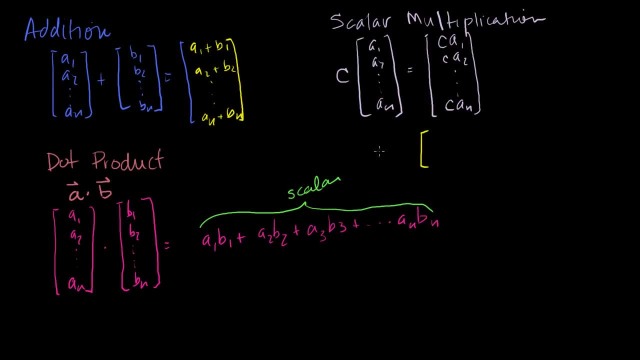 So let's say that we take the dot product of the vector 2, 5, and we're going to dot that with the vector 7, 1.. Well, this is just going to be equal to 2 times 7, plus 5. 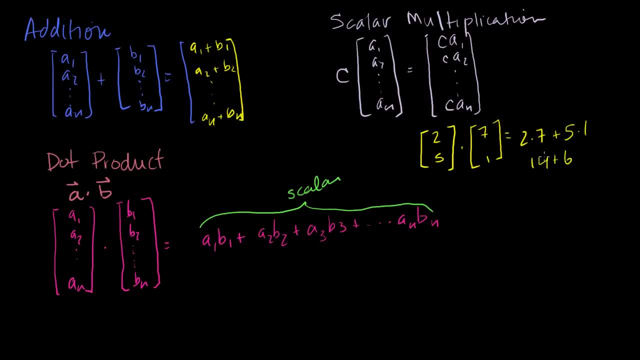 times 1, or 14 plus 6.. No, sorry, 14 plus 5,, which is equal to 19.. So the dot product of this vector and this vector, it's 19.. Let me do one more example, although I think this is a. 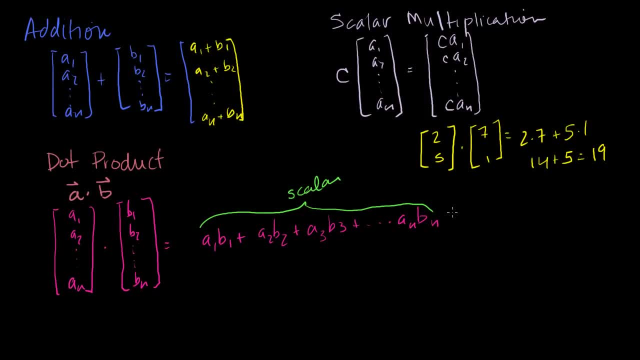 pretty straightforward idea. Let me do it in MOV. OK, so I have the vector 1, 2, 3, and I'm going to dot that with the vector minus 2, 0, 5.. So it's 1 times minus 2, plus 2 times 0,, plus 3 times 5.. 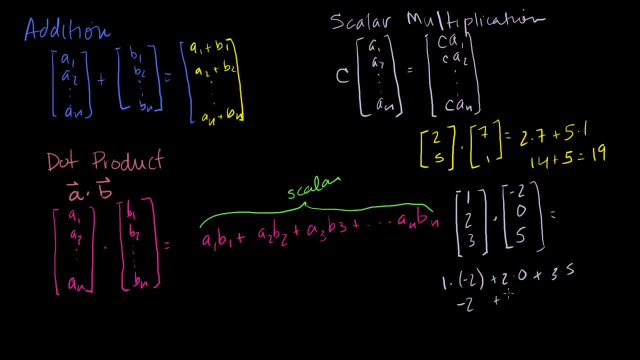 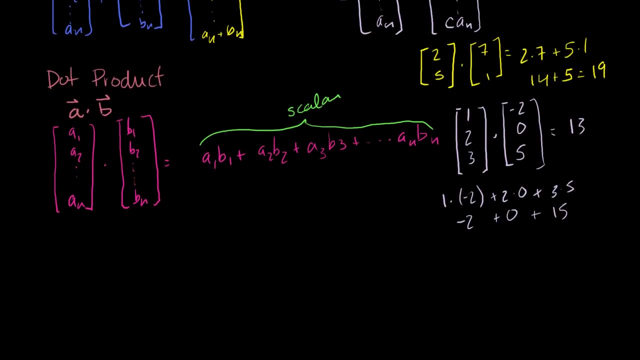 So it's minus 2, plus 0.. Plus 15.. Minus 2, plus 15 is equal to 13.. That's the dot product by this definition. Now I'm going to make another definition. I'm going to define the length of a vector. 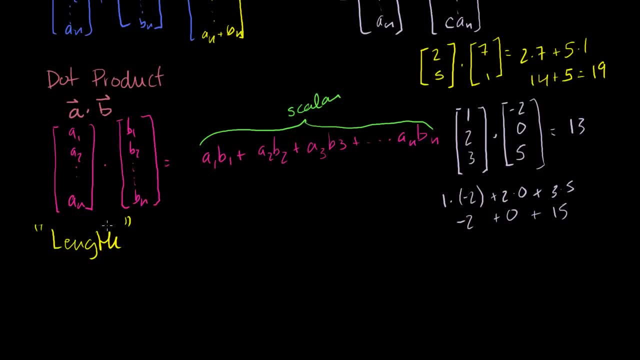 And you might say, Sal, I know what the length of something is. I've been measuring things since I was a kid. Why do I have to wait until a college level? or hopefully, you're taking this before College, maybe, but what is now considered a college level? 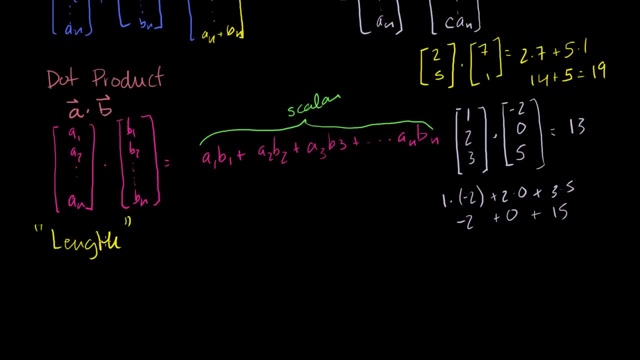 course, to have length defined for me, And the answer is because we're abstracting things to well beyond just R3, or just three-dimensional space is what you're used to. We're abstracting that these vectors could have 50 components And our definition of length will work even for these 50. 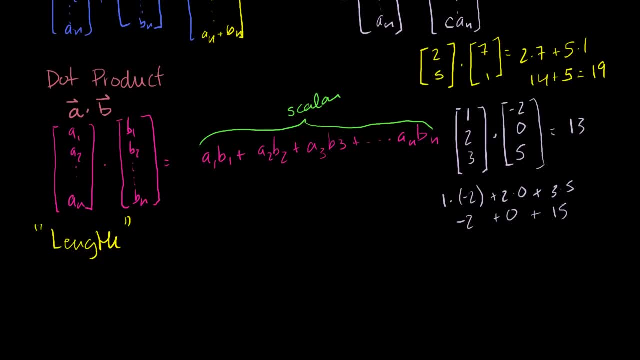 component vectors, And so my definition of length. but it's also going to be consistent with what we know length to be. So my definition. so if I take the length of a, and the notation we use is just these double lines around the vector. 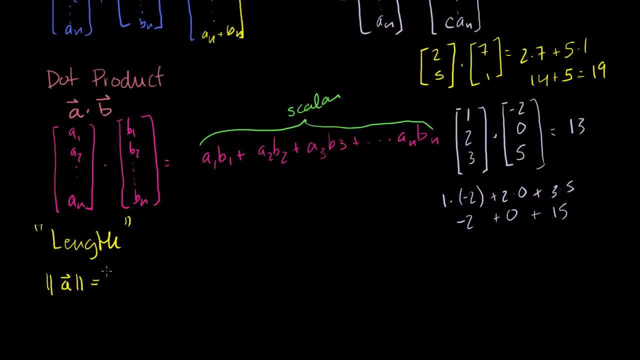 The length of my vector a is equal to- and this is a definition. it equals the square root of each of the terms, each of my components, squared, added up Plus a2, squared plus all the way to plus an squared, And this is the definition. 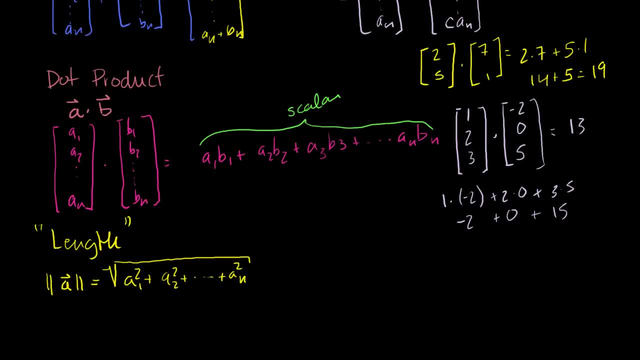 So if I take the length of a and the notation we use is just these double lines around the vector, the length of my vector squared, And this is pretty straightforward. If I wanted to take the let's call this, this was vector b. 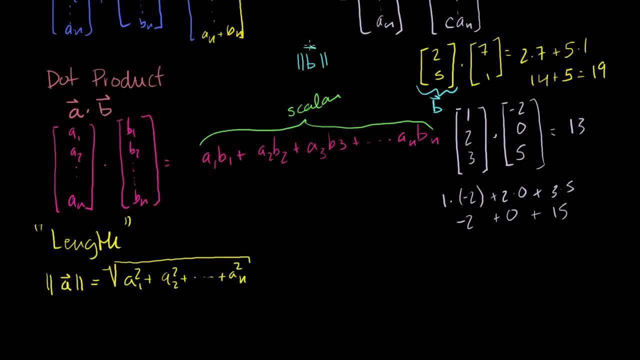 If I wanted to take the magnitude of vector b right here, this would be what. This would be the square root of 2 squared, 2 squared plus 5 squared, which is equal to the square root of what is this: this is 4 plus 25, the square root of 29.. 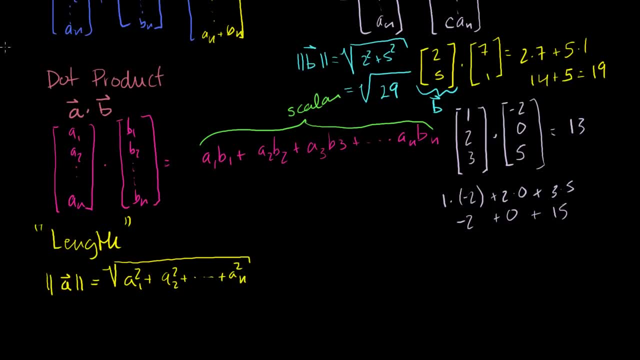 So that's the length of this vector And you might say: look, I already knew that That's from the Pythagorean theorem. If I were to draw my vector b, let me draw it. Those are my axes. My vector b, if I draw it in standard form, looks like. 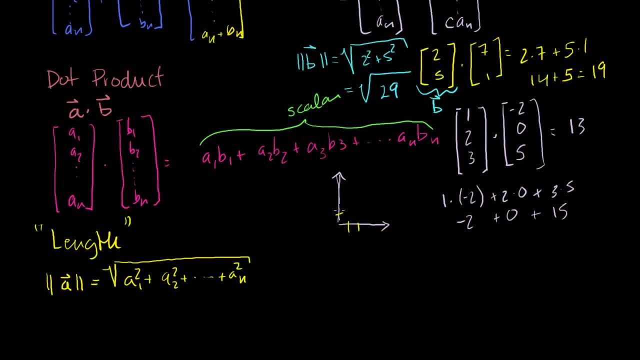 this: I go to the right- 2,, 1,, 2, and I go up 5.. 1,, 2,, 3,, 4,, 5.. So it looks like this. My vector b looks like that: 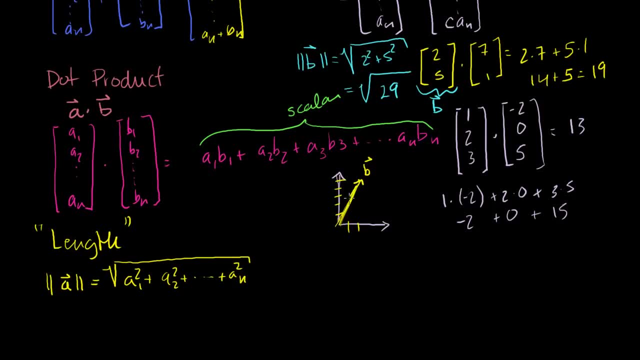 And from the Pythagorean theorem. you know, look, if I wanted to figure out the length of this vector in r2, or if I'm drawing it in kind of two-dimensional space, I take this side which is length 2, I take that side which is. 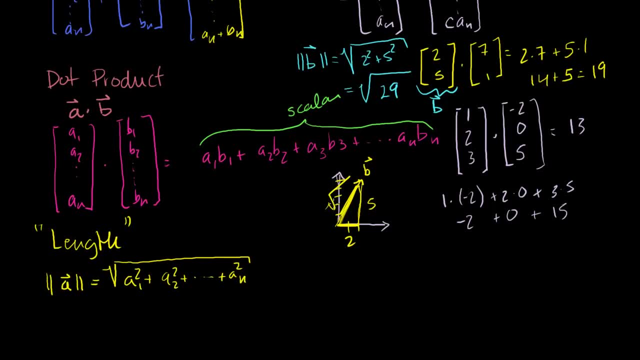 length: 5,. this is going to be the square root from the Pythagorean theorem of 2 squared plus 5 squared, which is exactly what we did here. So this definition of length is completely consistent with your idea of measuring things in one, two or three. 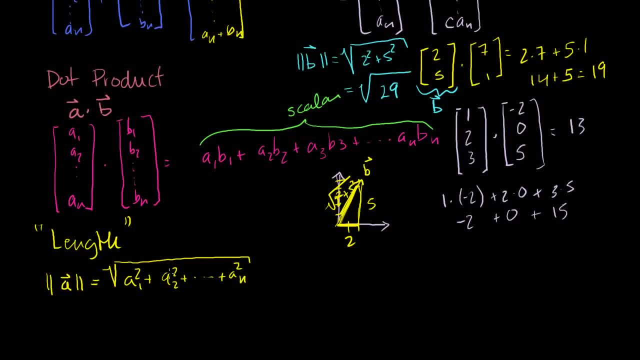 dimensional space. But what's neat about it is that now we can start thinking about the length of a vector that maybe has 50 components, Which you know, really to visualize it in our traditional way makes no sense. But we can still apply this notion of length and start to 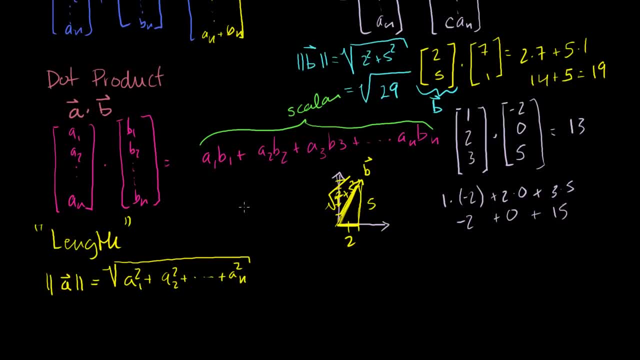 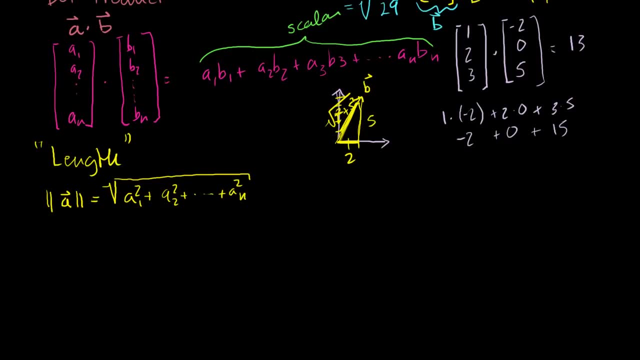 maybe abstract beyond what we could traditionally associate length with. Now can we somehow relate length with the dot product? Well, what happens if I dot a with itself? What is a dot a? So that's equal to. I'll just write it out again: a1, all the. 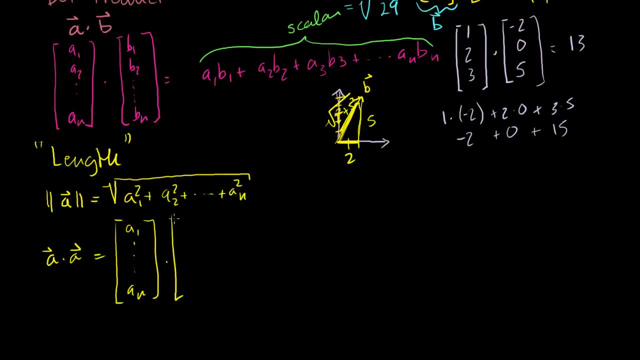 way down to an Dotted with a1, all the way down to an. Well, that's equal to a1 times a1, which is a1 squared plus a2 times a2, a2 squared plus all the way down. keep doing. 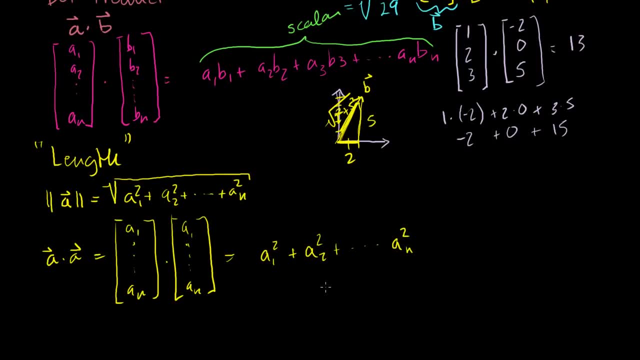 that all the way down to an times an, which is an squared. Well, what's this? This is the same thing as the thing you see under the radical. These two things are equivalent. So we could write our definition of length of: 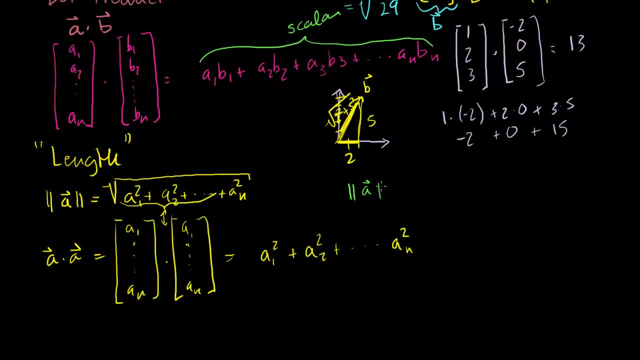 vector length, We can write it in terms of the dot product, of our dot product definition. It equals the square root of the vector dotted with itself. Or if we square both sides, we could say that our new length definition, squared, is equal to the dot product of a vector. 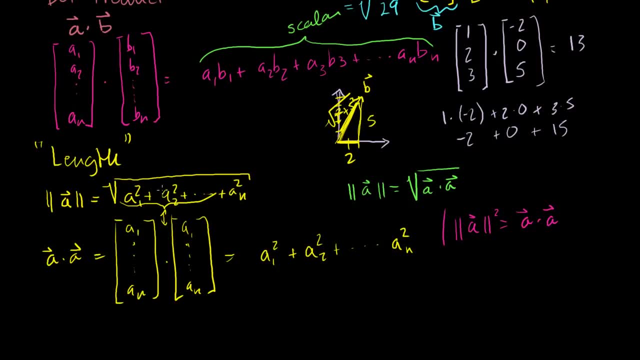 with itself And this is a pretty neat. it's almost trivial to actually prove it, but this is a pretty neat outcome and we're going to use this. We're going to use this in future videos. So this is an introduction to what the dot product is, what 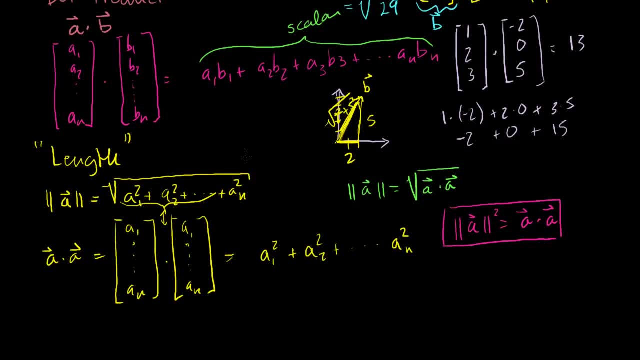 length is. In the next video I'm going to show a bunch of properties of it and it'll almost be mundane, But I want to get all those properties out of the way so we can use them in future proofs. 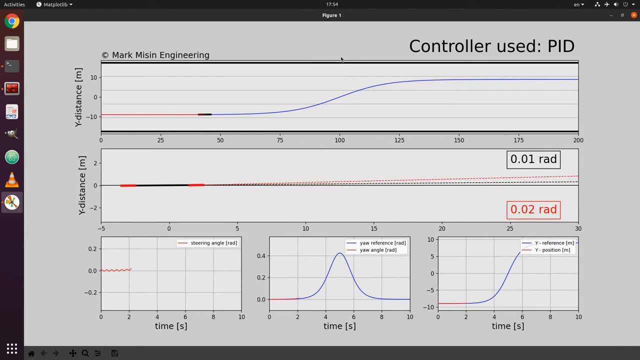 Welcome back. In this video I want to show you a vehicle that is driving on a straight road, attempting to change lanes. This is the vehicle right here. These are the lanes 1, 2,, 3,, 4 and 5.. The blue line is the reference trajectory that the